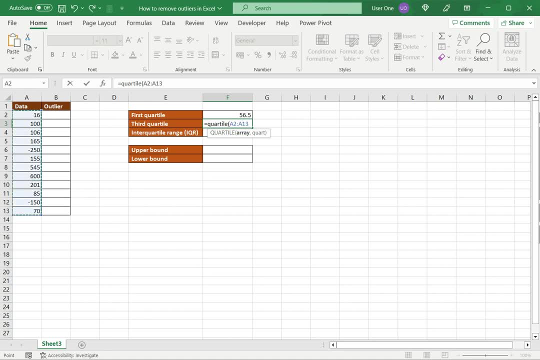 so again, we'll take the and specify number 3, because it's the third quartile. I then need to find the interquartile range, which is the third quartile minus the first quartile. So now I have the IQR. Now, using this IQR, I can define an upper and a lower bound. 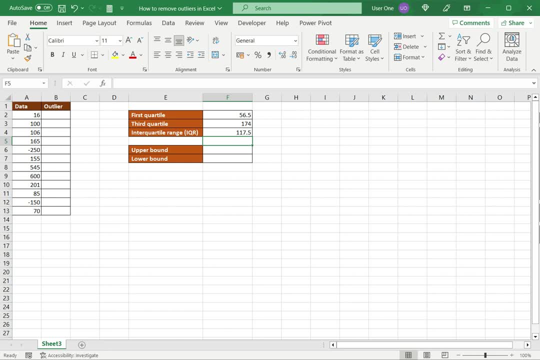 The upper bound is the third quartile plus 1.5 times the interquartile range. So it is the third quartile plus 1.5 into the interquartile range. This is my upper bound and the lower bound is the first quartile minus 1.5. 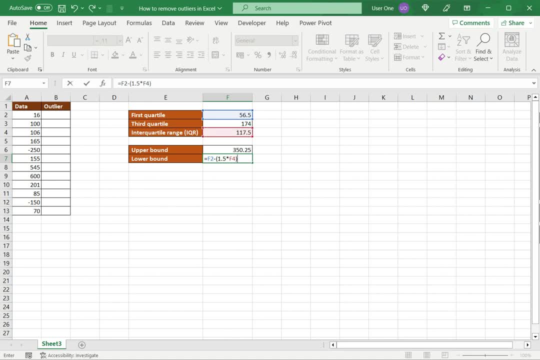 into the interquartile range And enter. So now I have an upper bound and lower bound. Now I'm going to compare each value against these two values, and whatever is either greater than the upper bound or lesser than the lower bound can be considered an outlier. 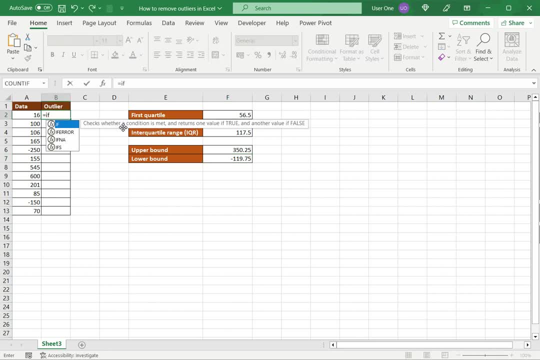 So to do this comparison, I will use the IF function. Now, IF takes a logical test and returns a value if the test is true and another value if the test is false. Now in this test, I want to check if the value falls outside the upper bound. 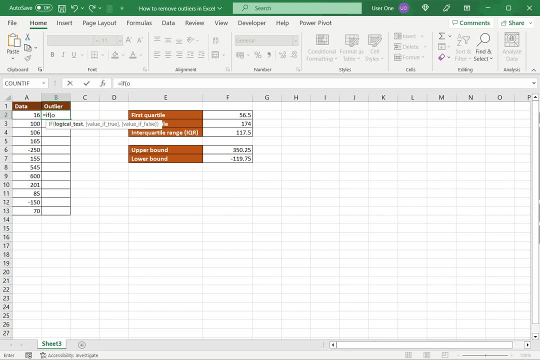 or outside the lower bound. So since there are two conditions, I will use the OR function, where I can define two cases. So here, the first case is whether the data is lesser than the lower bound, Or the second case is if the data is greater than the 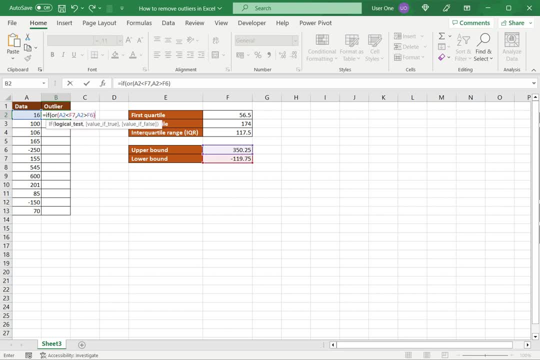 upper bound. So the OR function will check whether either one of these are true. So if this is true, I want it to say true, And if it is not, I want it to say false, Meaning that if it falls outside these limits. 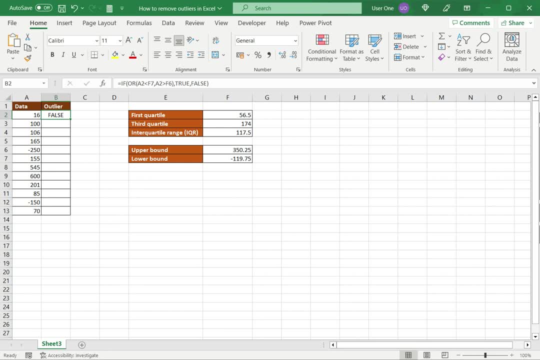 it is an outlier, otherwise it isn't, And say enter: So in this case it is false. It is not an outlier Because 16, I mean, if you look at it- does fall between these. Now, before copying this down, I need to make the upper and lower bound constant. 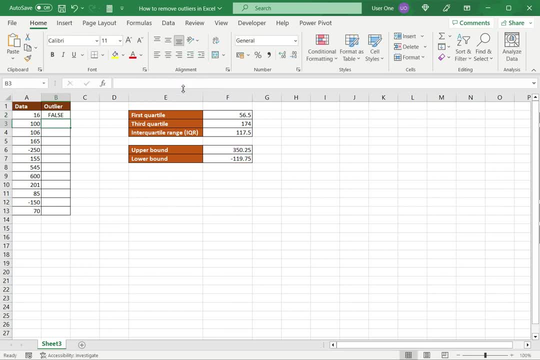 So I'll select the cell reference and press F4.. Now I can copy the formula by just dragging it down and straight away I can see my outliers are displayed and now I want to remove them. So I will go to the data tab and say filter.